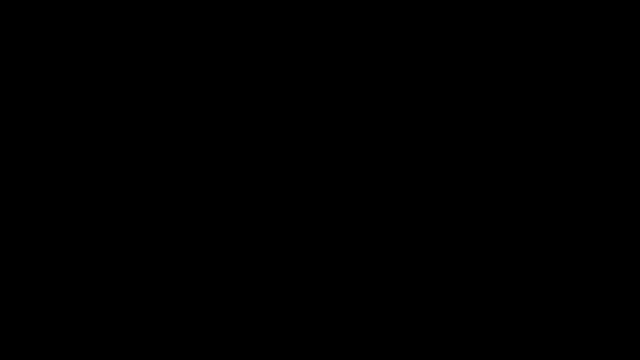 In this video we're going to talk about how to simplify rational expressions when adding or subtracting them whenever they have like denominators. So let's start with this example: 3x over 5 plus 4x plus 7 over 5.. 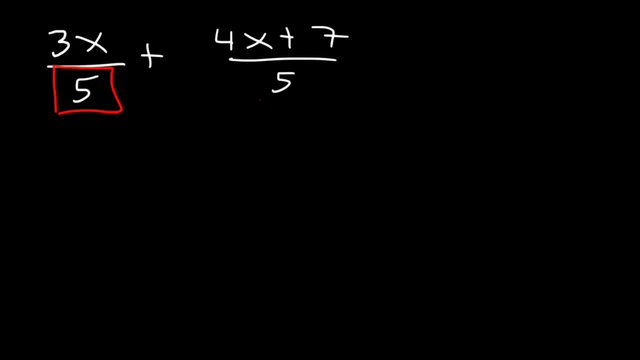 Because these two fractions share the same denominator, we can combine it as a single fraction. So we can write it as 3x plus 4x plus 7, all divided by the common denominator, which is 5.. 3x plus 4x is 7x. 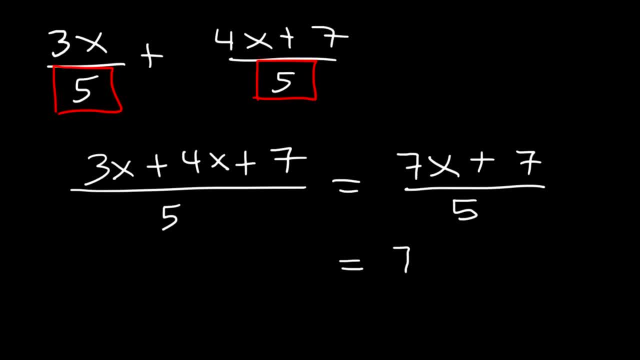 And, if we want to, we can take out the GCF, which is 7, leaving behind x plus 1.. So that's the final answer for this example. Let's try another one: 7 over x minus 11 over x. 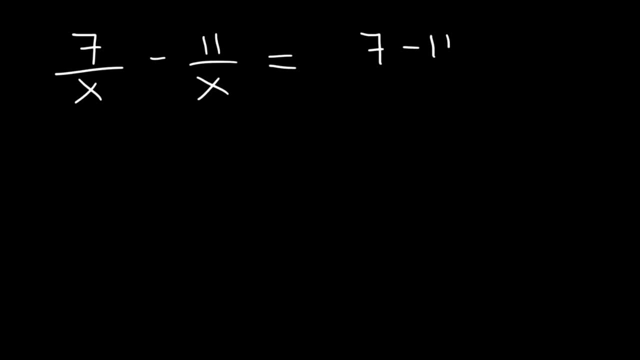 So we can combine it as a single fraction: 7 minus 11 over x, And 7 minus 11 is negative 4.. So the answer is going to be negative 4 divided by x. Try this one: 7x plus 4 divided by x plus 2, plus 5x minus 7 over x plus 2.. 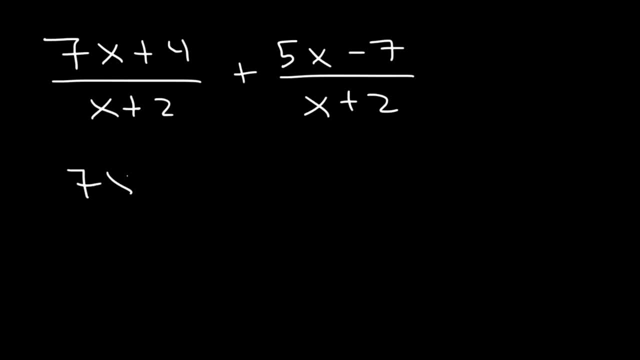 So let's write it as a single fraction: 7x plus 5x. I'm going to put the like terms together: plus 4 minus 7,, all divided by x plus 2.. 7x plus 5x is 12x. 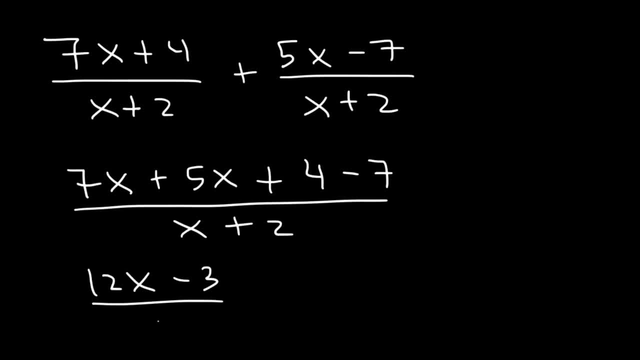 4 minus 7 is negative 3.. So we can take out a 3 if we want. So it's going to be 4x minus 1 over x plus 2.. And so that's it. Let's try one more example. 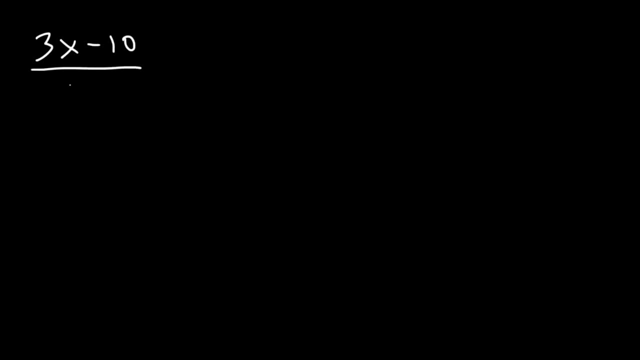 3x minus 10, divided by x minus 1 minus 5x minus 12, over x minus 1.. Now be careful with this one. Go ahead and try it. So first let's write it as a single fraction. So it's going to be 3x minus 10..